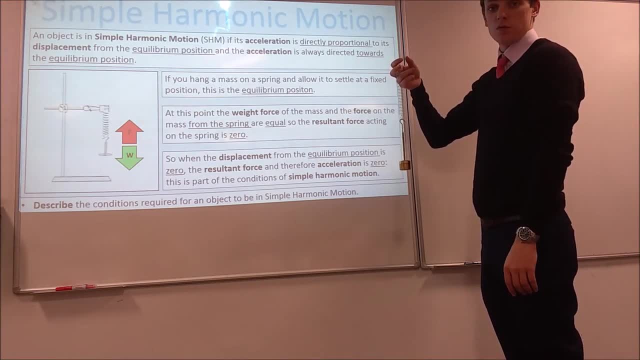 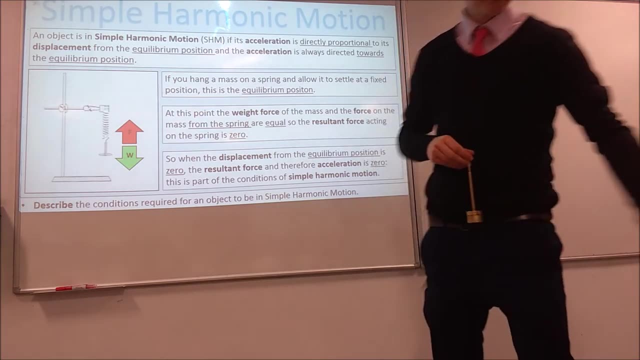 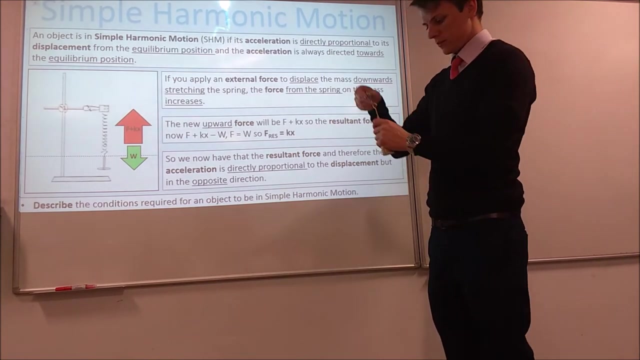 in this situation, its acceleration is zero because the resulting force is zero. So that's our first scenario there where it's not even oscillating at all. So let's have a look at what happens if we displace it downwards. Now, what we've got is: what do I mean by that? So this was its equilibrium position. Let's 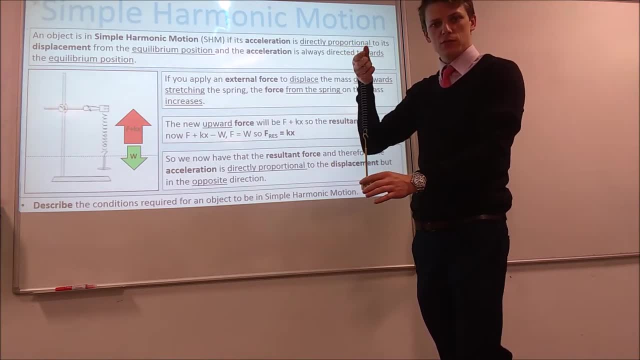 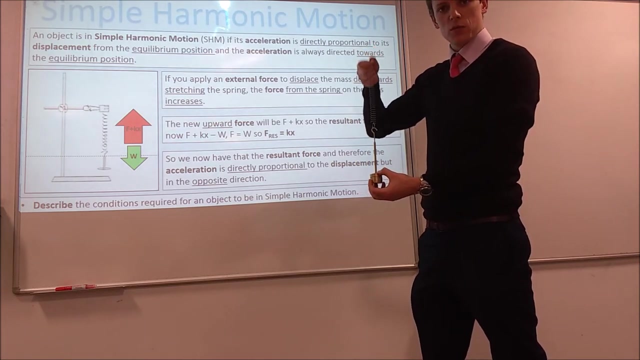 displace it downwards, And I do that by applying an external force to move it to that position, And then what I'm going to do is release it so that external force is no longer a factor. So we can see here that, having extended the spring, when I release this, the upward force, 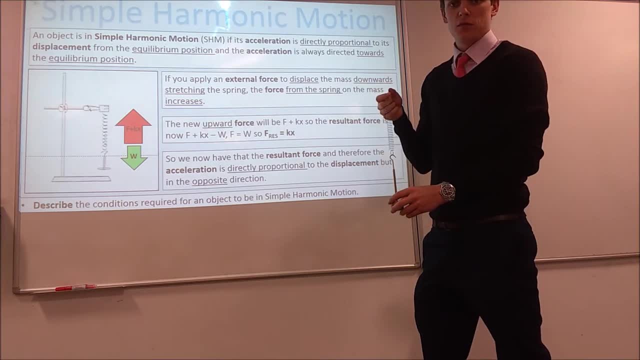 from the spring is going to be bigger than the downward force of the weight. Why? Because we've stretched it out. So if we calculate the increase in force from spring, it's going to be equal to k times the amount I displace it. 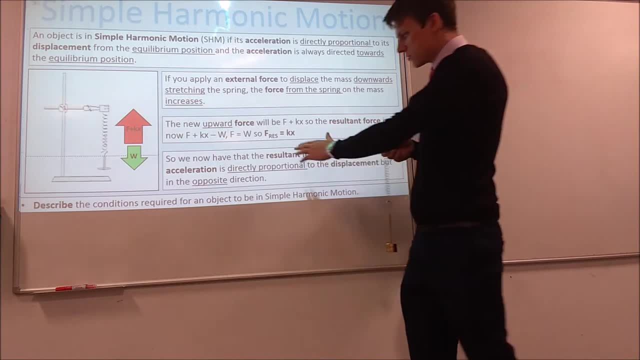 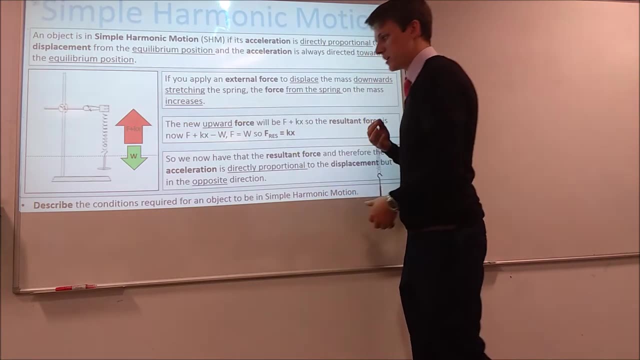 So now the resultant force acting on the object is going to be equal to k times x, because the weight force and the original force are going to cancel each other out. The resultant force is just going to be kx, using Hooke's law, And so what we can see from that is if the resultant force is directly proportional to. 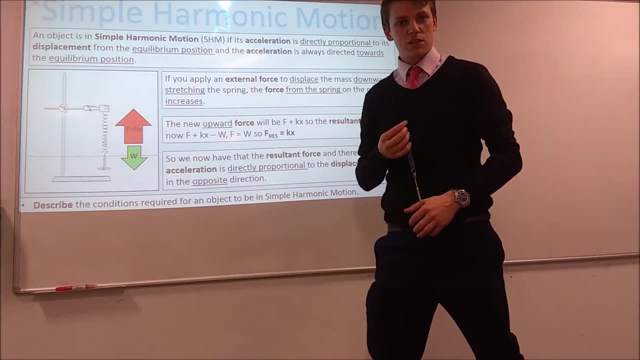 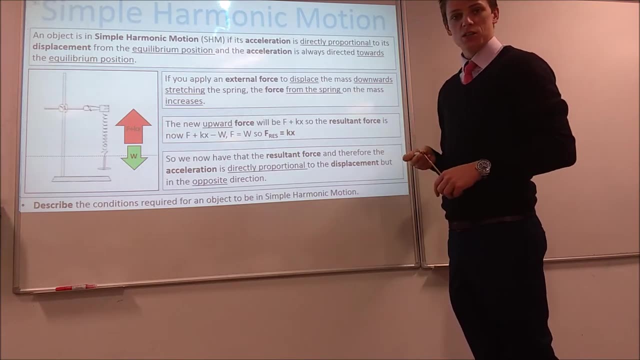 the displacement from the equilibrium position, then so is the acceleration going to be. So we've got that if we displace it downwards, the acceleration and the displacement are directly proportional. And if we think about the direction of the force, if I displace, 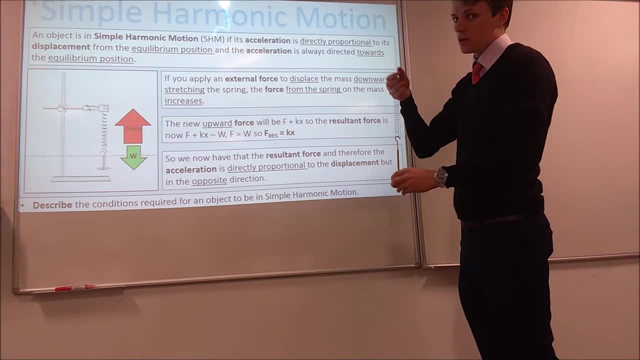 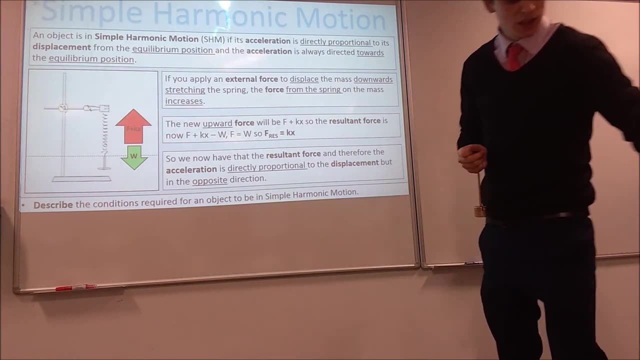 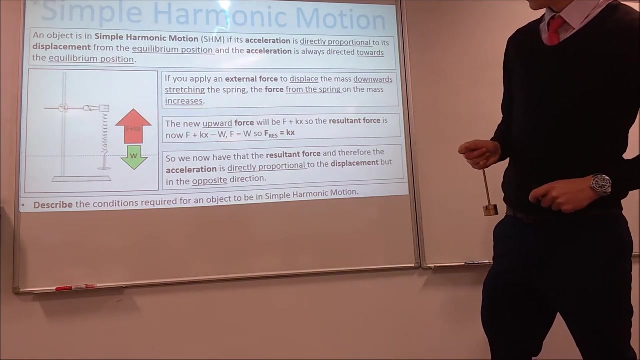 it downwards, then the force is upwards. So again in the opposite direction, the force is towards the equilibrium position. So that works if we displace it upwards. So let's try it if we displace it upwards as well. OK, so here's our equilibrium position. So if we apply an external force now to displace, 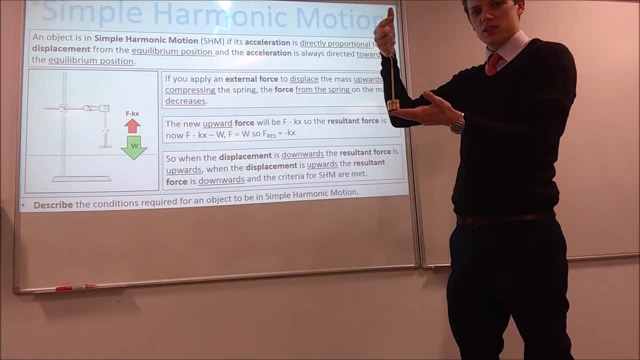 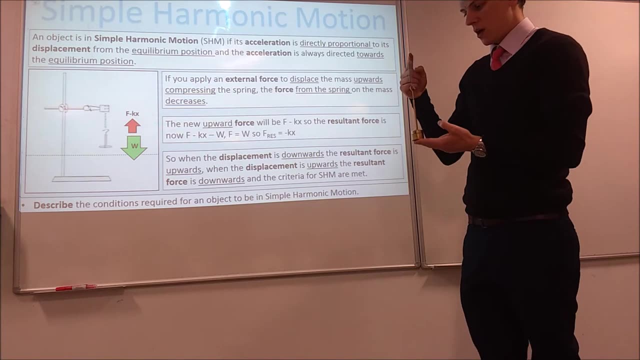 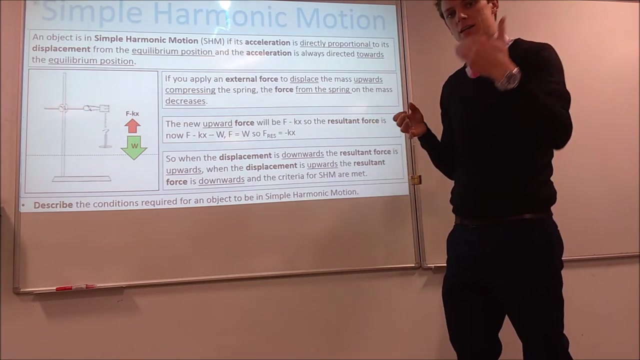 it upwards. what we've done is decrease the extension of the spring. So we've decreased the upward force, meaning the resultant force is now downwards, And we've decreased the upwards force by an amount- kx, So now the resultant force I would say is minus kx. 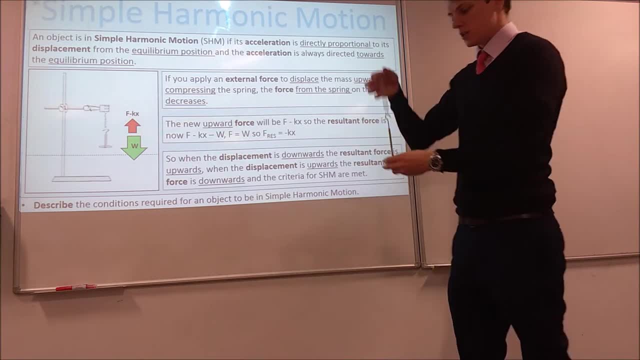 because it's in the opposite direction to what we had before. So we've got the resultant force of minus kx. The resultant force is downwards, the mass upwards. The resultant force is downwards, back towards the equilibrium position. So again in the opposite direction to displacement. 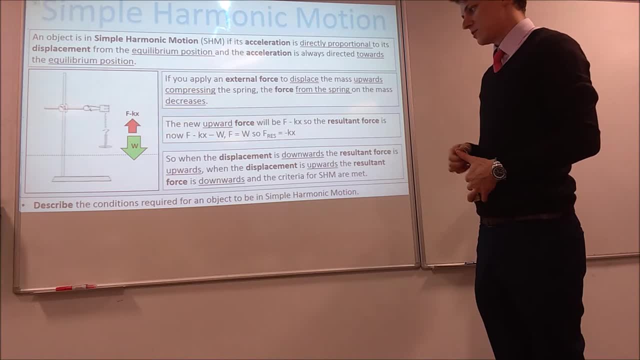 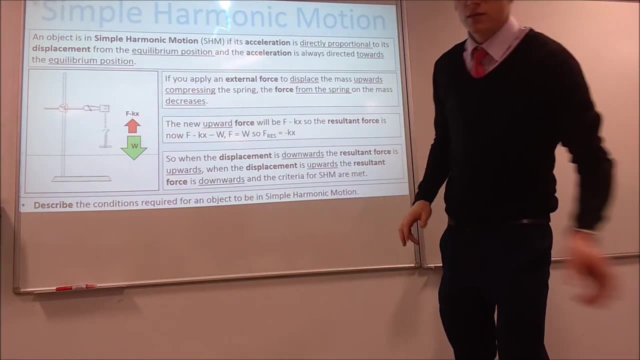 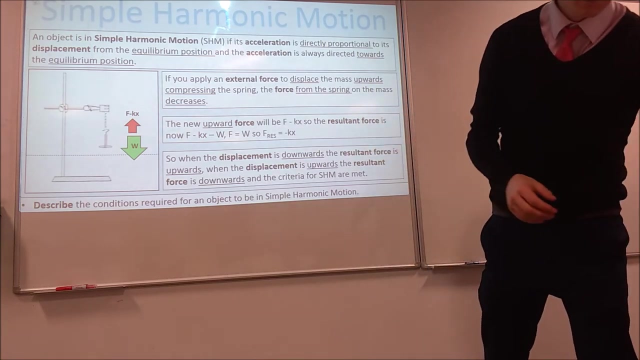 and again directly proportional to the displacement. So we've got our conditions of SHM shown there by this system in the three different positions. it can be above, below and at the equilibrium position. This is in SHM. So in terms of what that looks like, I realise I haven't actually shown you what SHM looks. 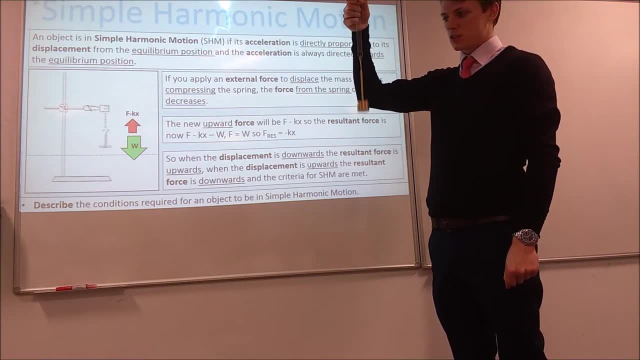 like: Essentially, this is SHM, It's just us. It's going to be oscillating, in this case, upwards and down with springs. Sometimes you get it sideways as well, But this is essentially what it looks like and it's oscillating about the equilibrium position. 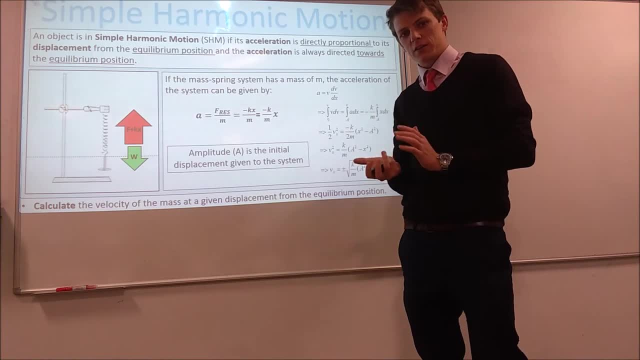 OK, so what we're going to look at now is some of the calculus that we can use to derive the equations we use to model an object in SHM. So the derivation process for this is not part of the A-level course, But any of you thinking of going on to do like maths, physics or engineering. 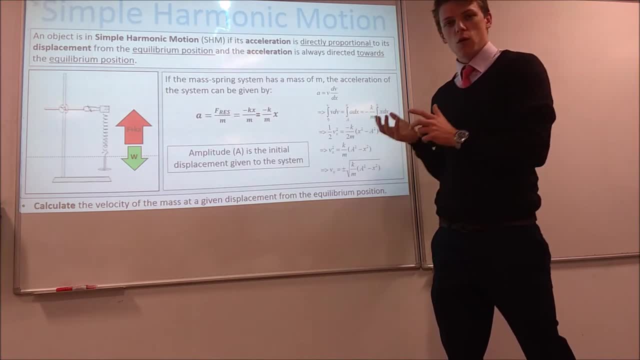 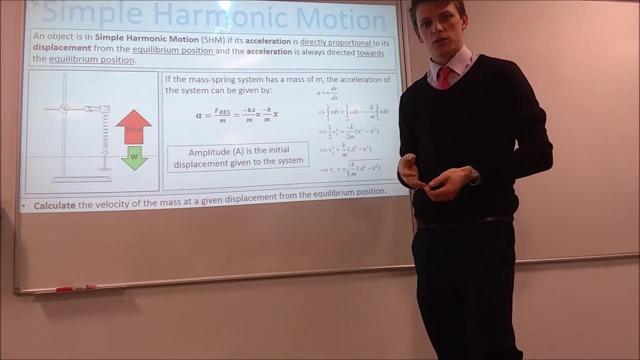 stuff should really pay attention to this, because this is really what you'd get into at that kind of level. So let's get through it and then the end result is realistically what you need for this part of the course, and we'll have a look at that in a minute. 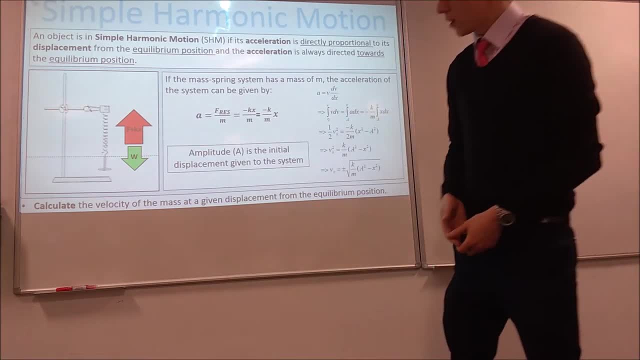 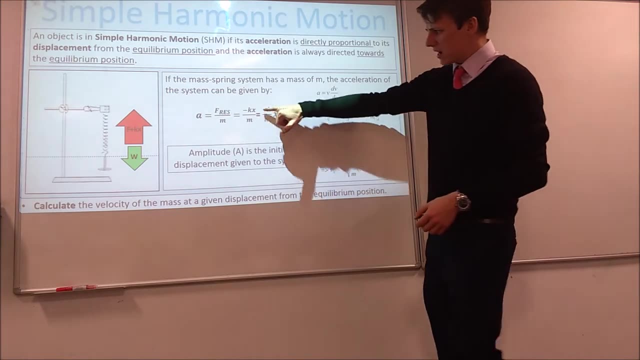 So we're going to take the example we were looking at before, where we displaced the object downwards. so we know the resultant force is directed upwards And we calculated it. if we define the downwards direction as positive, we know the resultant force is going to be. 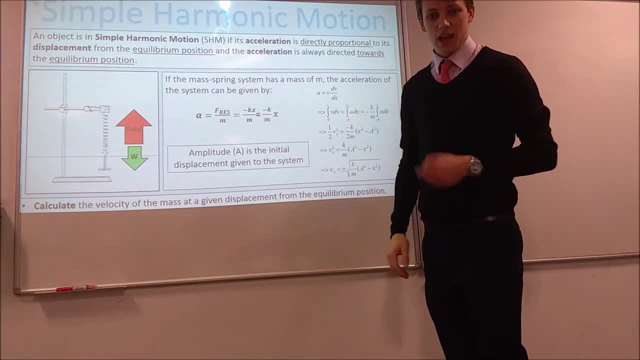 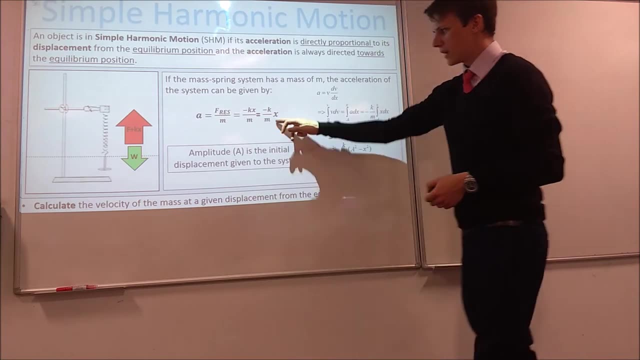 negative or in the upwards direction, and it's going to be equal to kx. So hence the resultant force is minus kx here. If we divide resultant force by mass, we will end up with acceleration. So we can get an expression for the acceleration in terms of the spring. 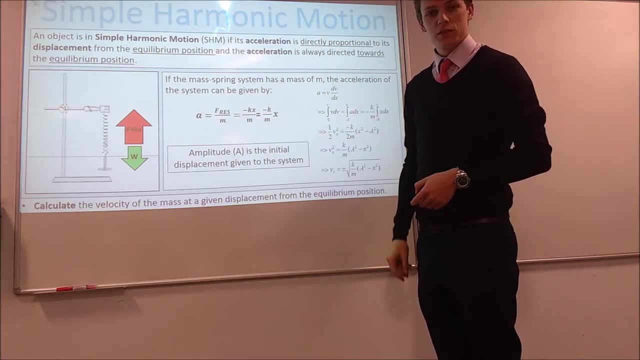 constant in terms of the mass of the system and of the displacement of the object from the equilibrium position. Now, those of you who get on to do symbols, you might be thinking that is just a expression of the mass of the feliz and the mass of the equilibrium. But, frankly, for us this is a 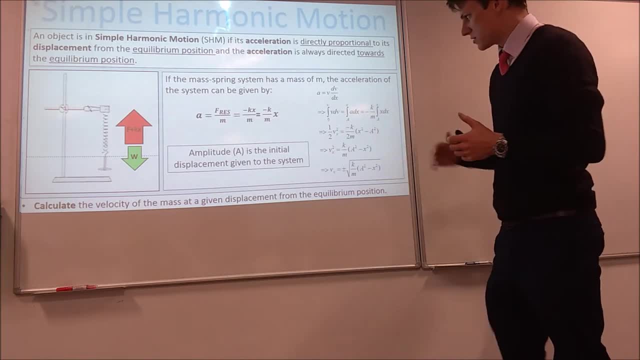 very common method, Because we're going to be using these equations to go on and on about the equilibrium and the mass of the equilibrium, And so we're going to take a moment to do the equation. then we're going to M2 and M3, the mechanics modules in maths will come across this relationship here. 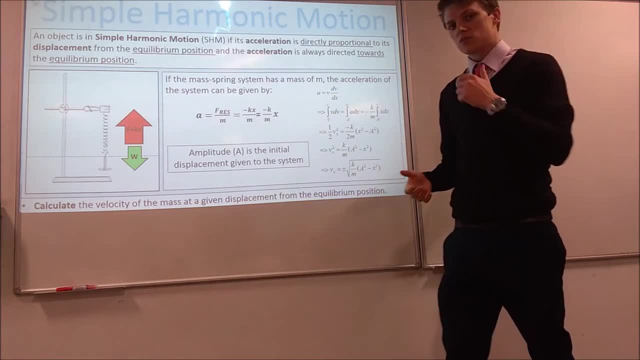 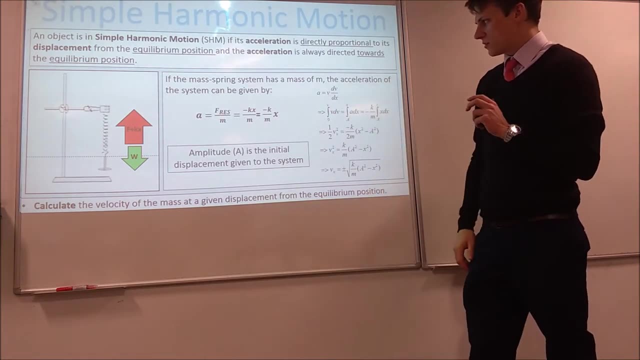 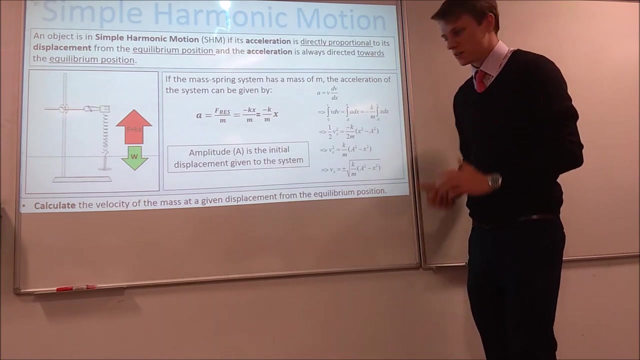 Essentially, you can calculate acceleration not just as the rate of change of velocity, but you can also do it using this expression: the velocity multiplied by the differential of velocity with respect to displacement. And we can check that that works by thinking about the units involved. 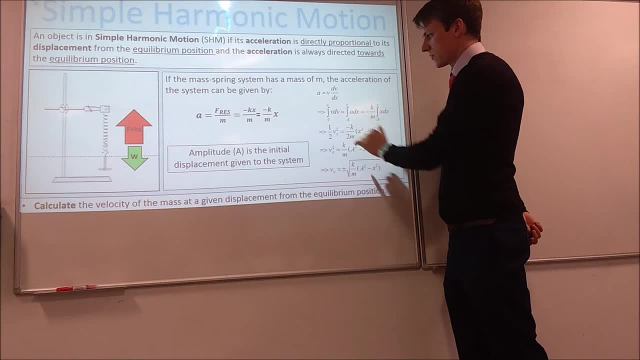 So velocity has a unit of metres per second. A change in velocity also has the unit of metres per second. So what we've got at the moment is metres squared s to the minus 2.. We're going to divide that by change in displacement metres, so we've got metres per second squared. 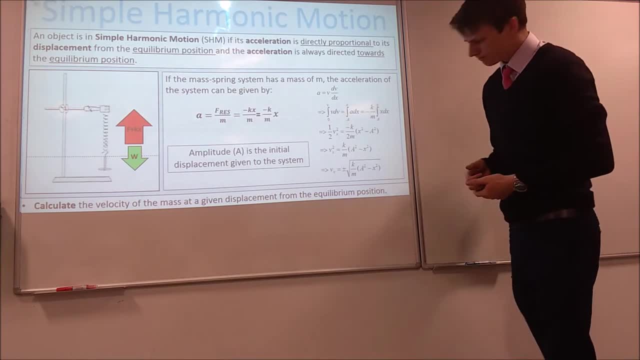 So you can see this expression works in terms of units. So what we're going to do is we're going to move the dx over to the other side, And the way we get rid of those partials is by integrating. So now we need to think about what that means. 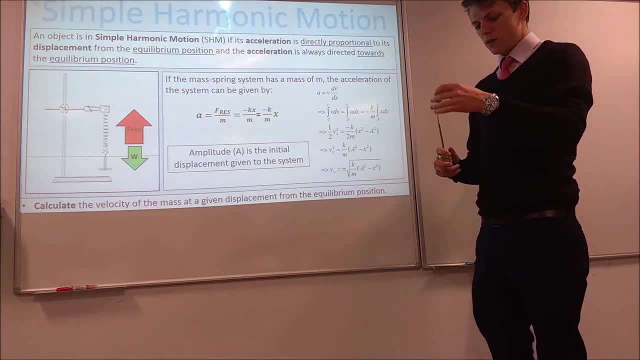 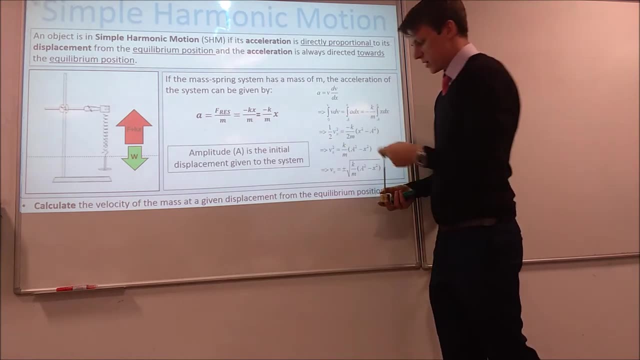 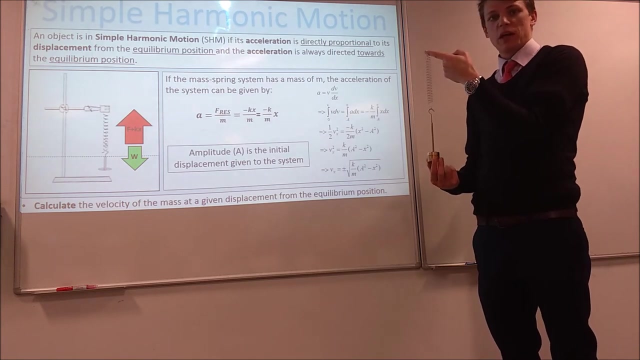 What the limits of our integration are here. So when we displace the object down, we can see it starts at a velocity of 0. So we're going to put the first limit of the integration with velocity as 0. It also starts at its maximum displacement, which is known as the amplitude. 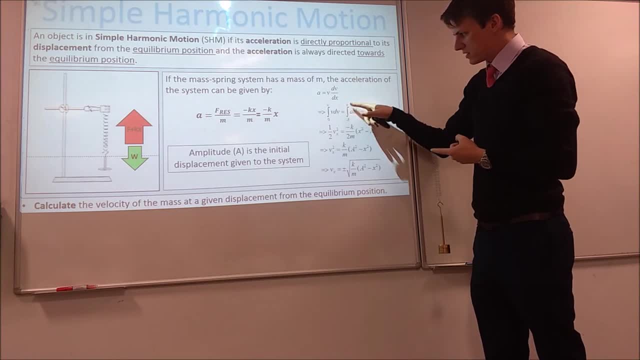 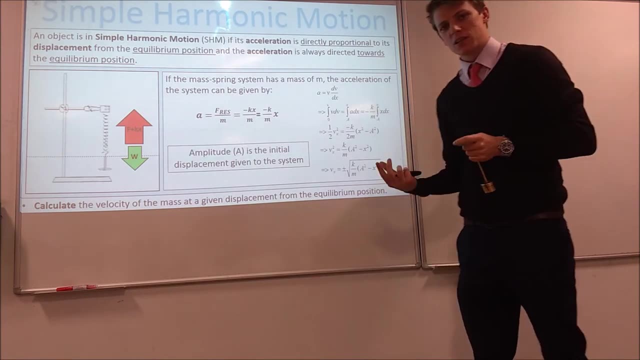 So we're going to start the integration with respect to distance at the amplitude here. OK, so where's it going to end up? Well, we want to know what the velocity is At any given displacement, x. We don't know what x is yet, so then we'd use that x to find v. 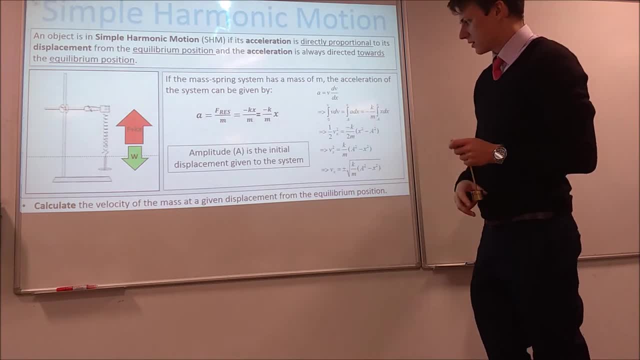 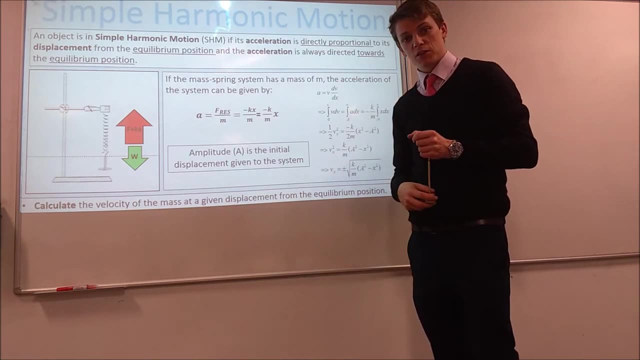 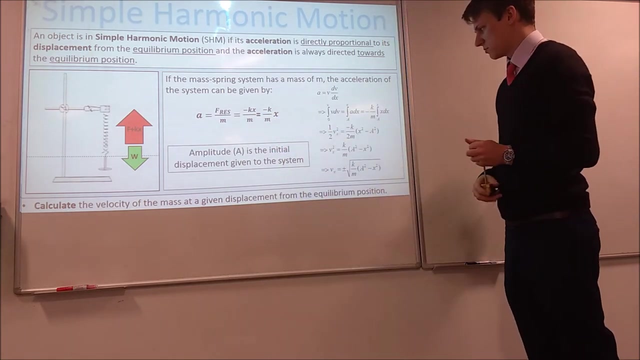 So we're going to integrate between v and the velocity and x in where we're integrating with respect to the displacement. here, Acceleration isn't a function of displacement at the moment. So what we're going to do is substitute, in this expression we had here, for acceleration, which is a function of displacement. 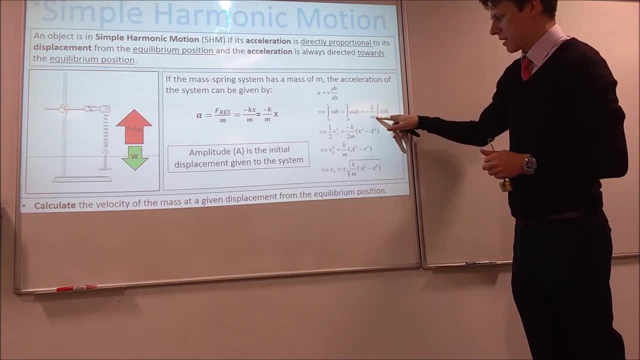 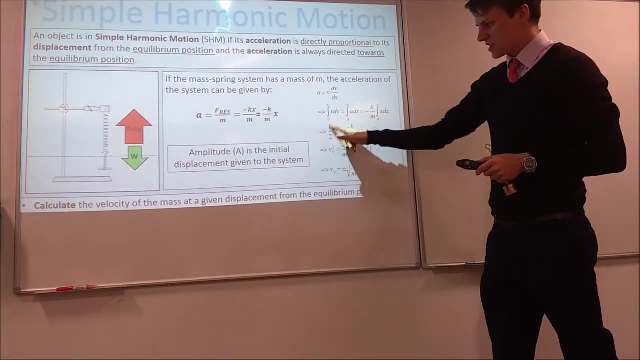 And that's what we've got here, And I've just taken all the minus km outside because those are all constants. So once we integrate, We can get this expression here and we can cancel out the halves, And we can cancel out the minus sign in here and switch what's around in the brackets. 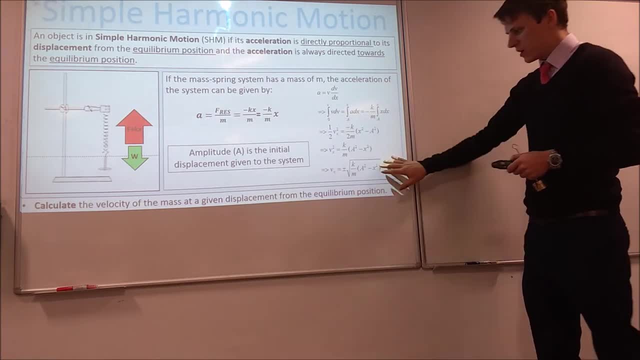 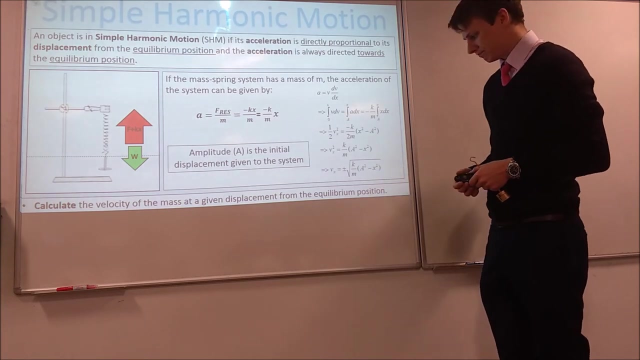 And then, finally, we can square root it at the end, to end up with this expression: for the velocity at a given displacement, x, And it's equal to the plus or minus square root of k over m multiplied by a squared: the amplitude squared minus the displacement squared, or x squared. 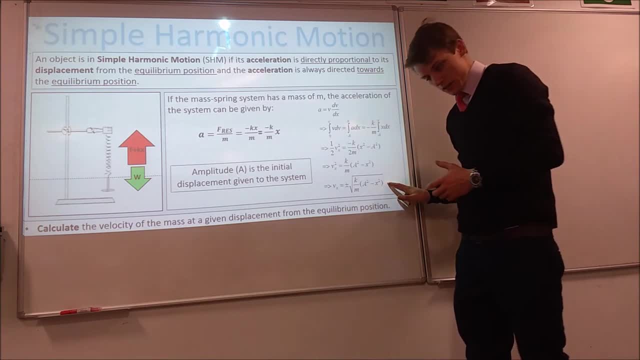 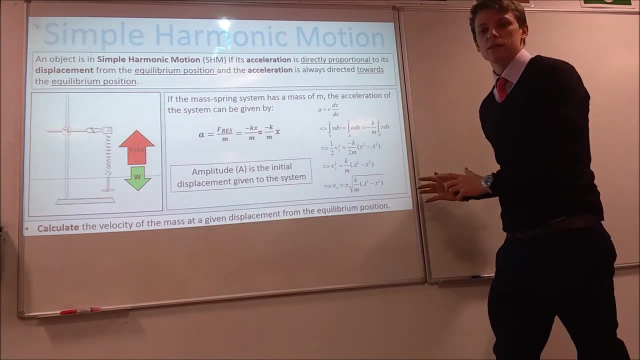 So, with this expression here, If you look in the formula sheets that you get, it's very, very close to one of them you get And we'll see in a minute how we can adjust it slightly to make it exactly the same. But before we can do that, we need to look at this SHM from a different perspective. 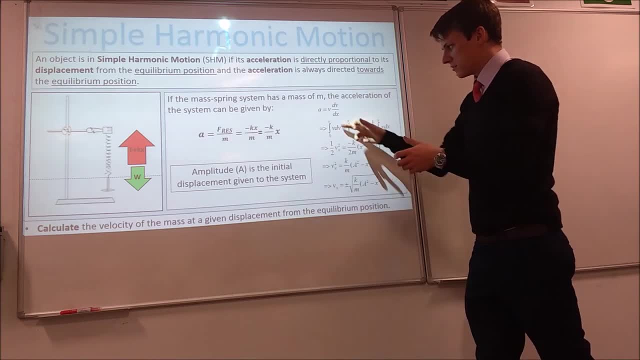 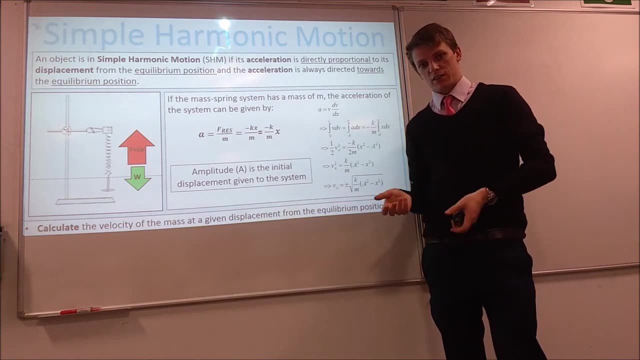 So we've looked at acceleration and we found essentially velocities at different displacements. But what if we want to find the velocity at a moment in time instead of at a fixed displacement? Well, we can do that. So what we're going to do is modulate. 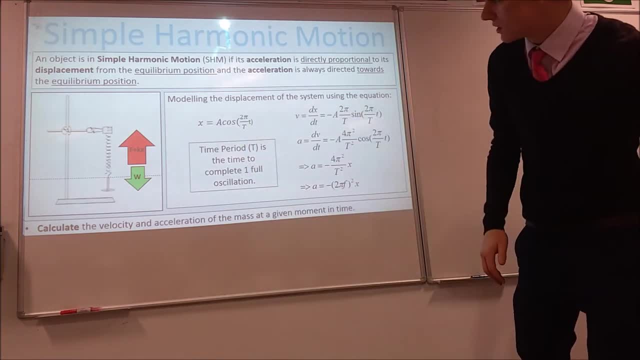 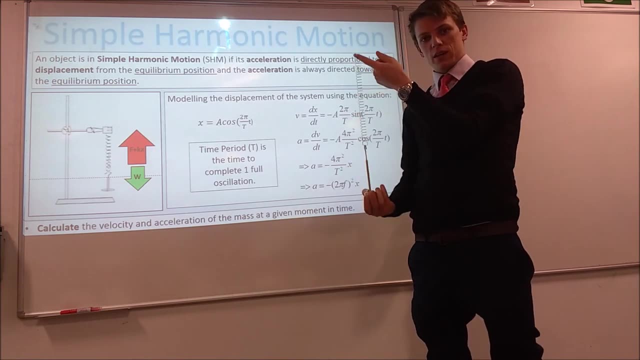 We're going to model the displacement using this cosine function here, So let's dig into how that works. So when we start an object oscillating, we're going to start it from its maximum displacement, because we have to give it an initial displacement. 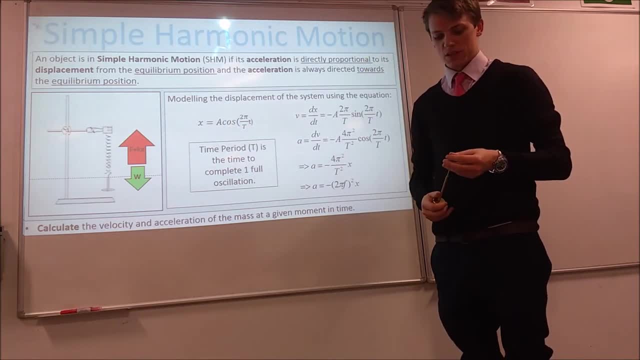 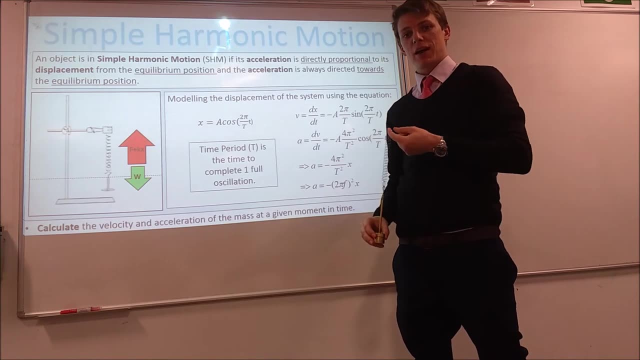 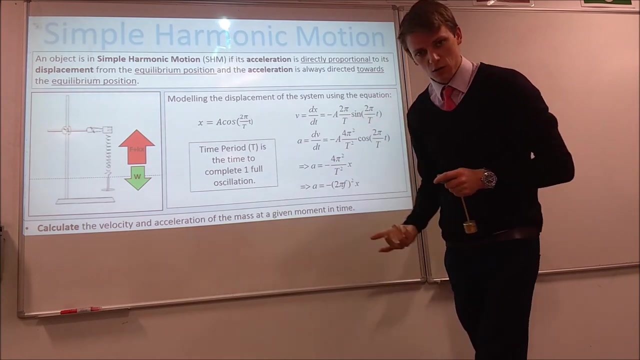 That's why we need a cosine function, because it's got to start at a maximum. at time equals zero. Then after one full time period it needs to go all the way up and all the way down back to maximum displacement. So the time over t here is to make it so after one time period it starts the whole cycle again. 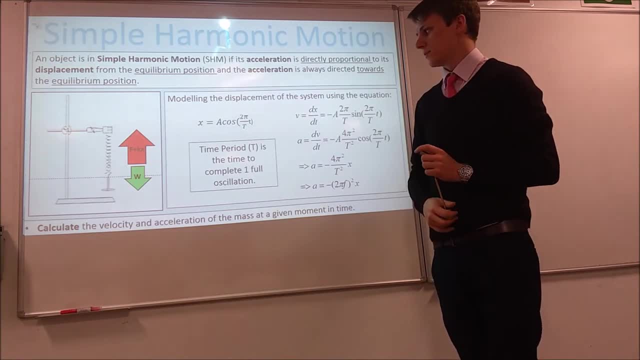 So time period is the time it takes to complete one full oscillation. So you can see, when we put in, t equals the time period, we get cosine of two, pi, which in terms of radians is back to the star again. And then finally, we need to make sure that at time zero the displacement is the amplitude. 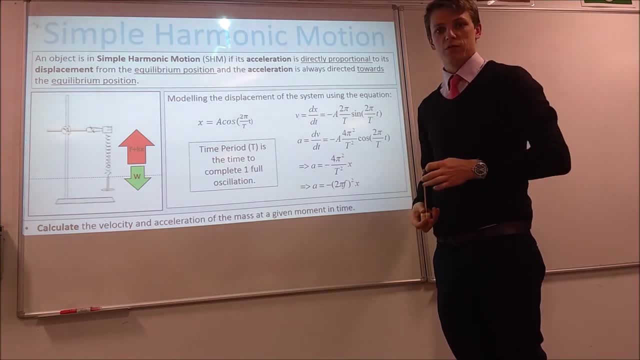 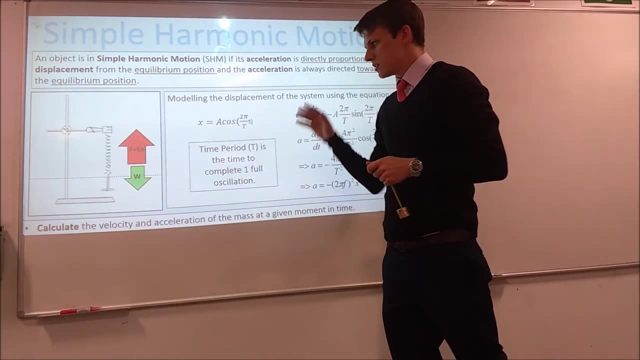 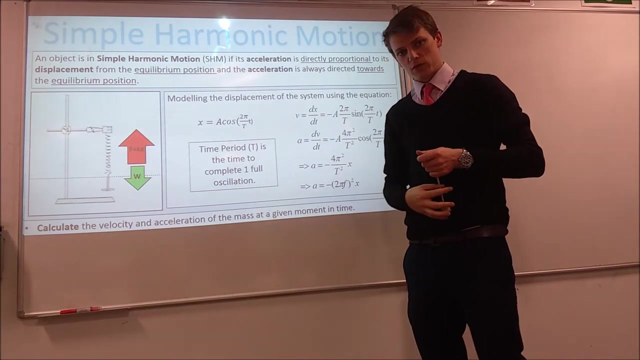 So we multiply the whole thing by the amplitude or the maximum displacement from the equilibrium position. So that's how we get displacement And, as you should know from your mechanics, before to go from displacement to velocity, what we need to do is find the rate of change of it, which is the same as finding the derivative with respect to time. 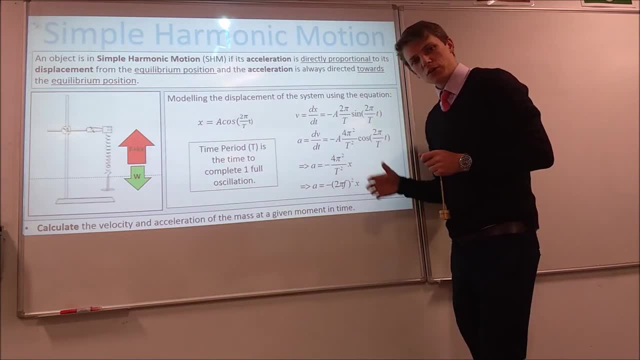 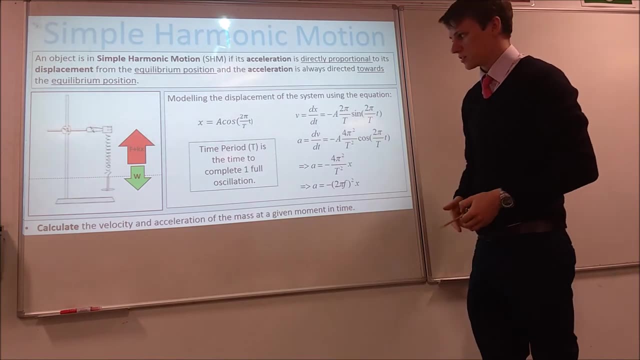 So that's what we're going to do here. So if you haven't got to this stage yet, in maths essentially you can. There are a set of ways to take the derivative of sine and cosine functions. So to go from a cosine function, the derivative is a minus sine function. 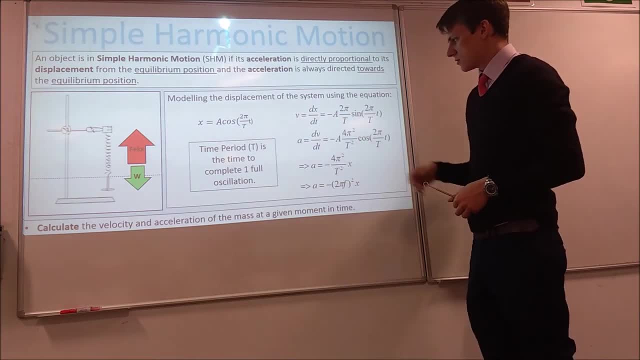 And in maths you'll explore why that's the case And so. So that's why I've got minus sine here. And what you also do is take whatever's multiplying by the t inside the function, You multiply that outside here. So that's why we get this expression here. 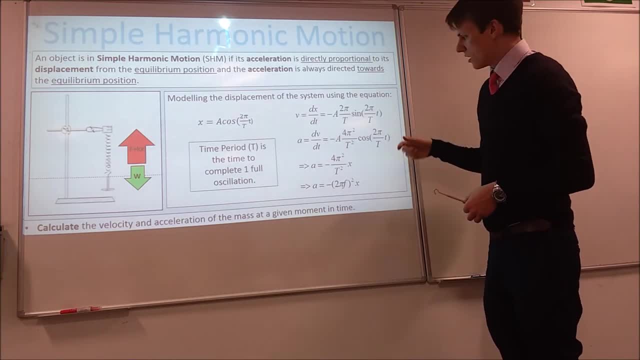 We can do the same process again to get acceleration, But a minus sine. take the derivative, you get a minus cosine function And again you take the two pi over t outside. So that's why we've got four pi squared over t squared. 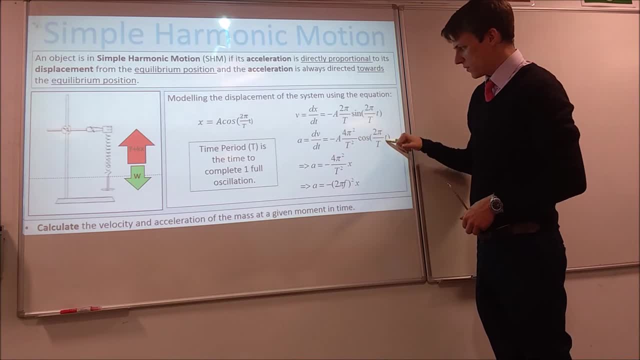 So what you notice here is a cosine two pi over time period times. t Is the displacement, So we can take all of that out and just put in its place displacement. And you can see, here we've got this sort of similar expression to what we had before. 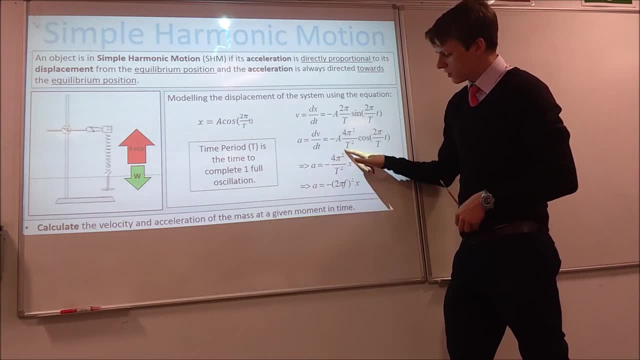 Acceleration and displacement are directly proportional. But we've got a different constant here And you should know that frequency is one over time period. So this is the most common way. you will see this expression right here in terms of two pi f squared as your constant. 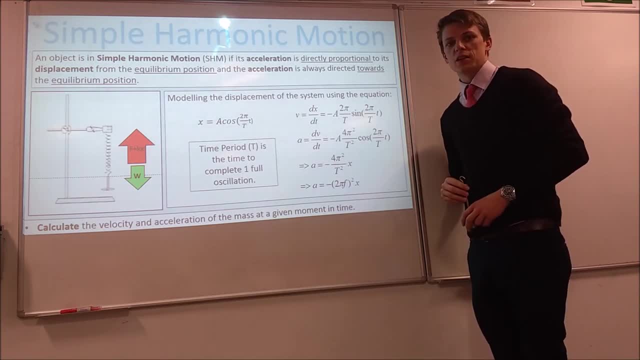 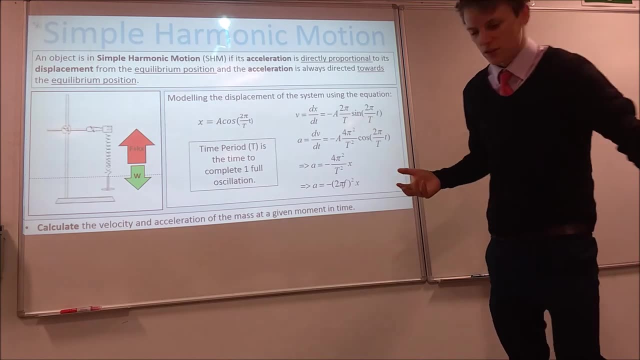 OK, So why have you gone through this process? Well, now it allows us to find a way of relating the time period of the frequency to the spring constant and the mass. So that's why this is useful. So let's have a look at that. 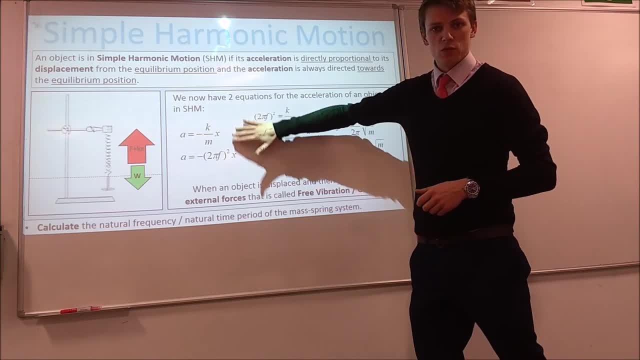 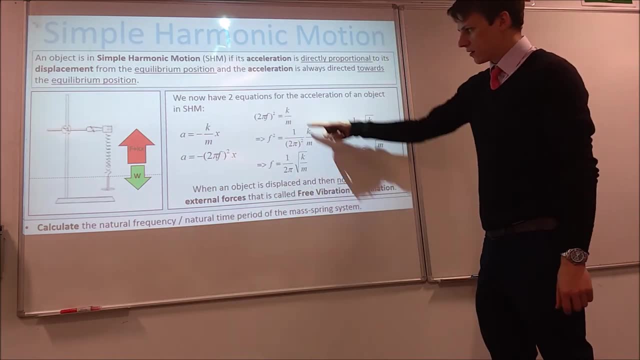 So we've got these two equations at the moment for the acceleration in terms of the displacement. So what we can do is equate the two constants together. that we've done here. Obviously, we don't need the minus signs. They cancel out. 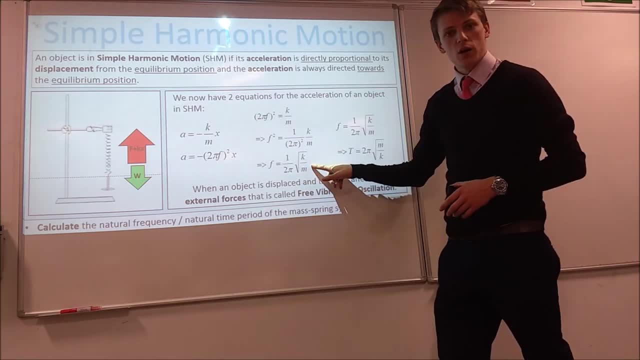 And we can rearrange to get an equation for the frequency. This is known as the natural frequency function. So this is the frequency of the system, or the frequency at which the system would oscillate if no forces are applied during the oscillation, or called free oscillation. 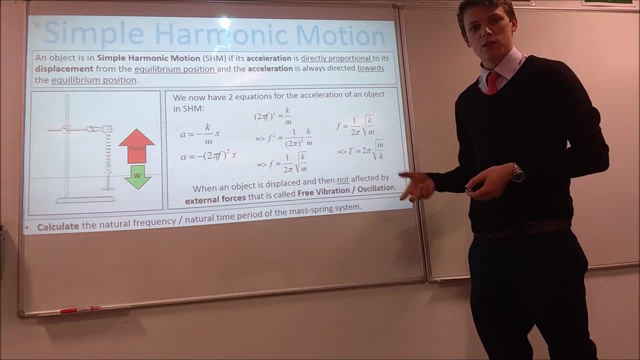 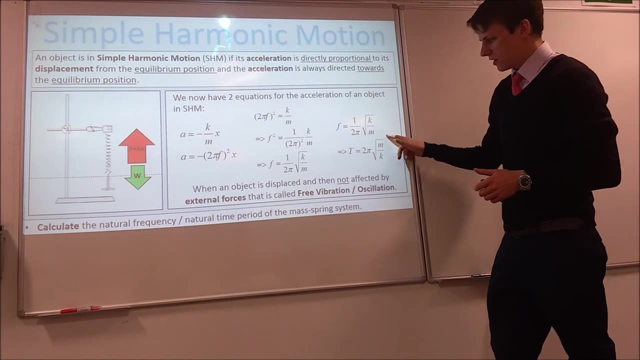 If we flip that whole thing over, we can get an expression for the natural time period or the time period of an oscillation, But again, when we're not applying any external forces to it, And that's this one here, And typically at a level, this is the one you see in your formula sheet here. 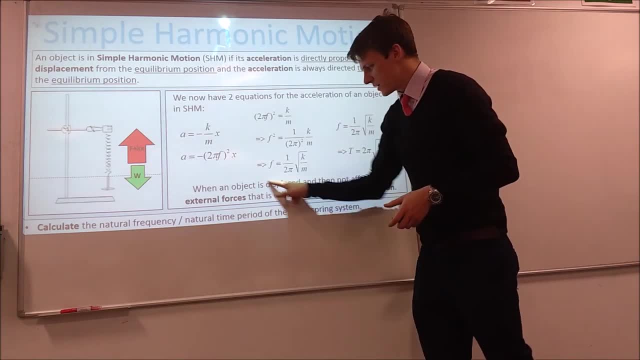 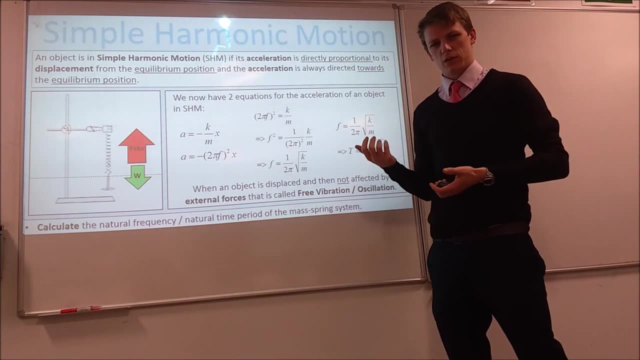 Once you get on to sort of like degree level- physics and engineering and stuff- you will more commonly see it in this form. So I don't know why a level insist on this one so much, Probably because you actually in your experiments time the oscillation. 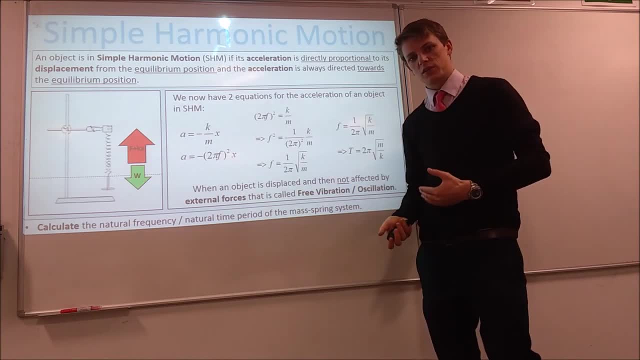 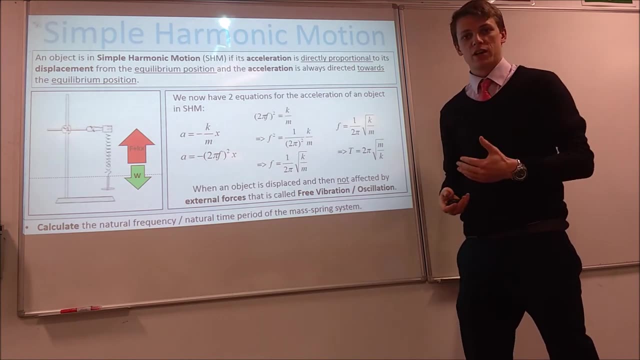 But we get these useful expressions to calculate what's called the natural frequency or the natural time period of the spring system when we set it oscillating in free vibration. OK, OK, So I'm going to finish up by summarizing the equation we've got. 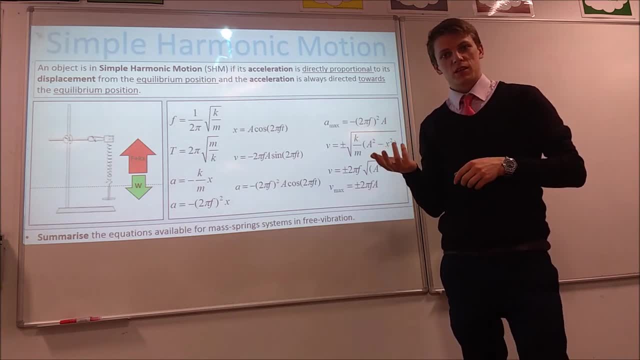 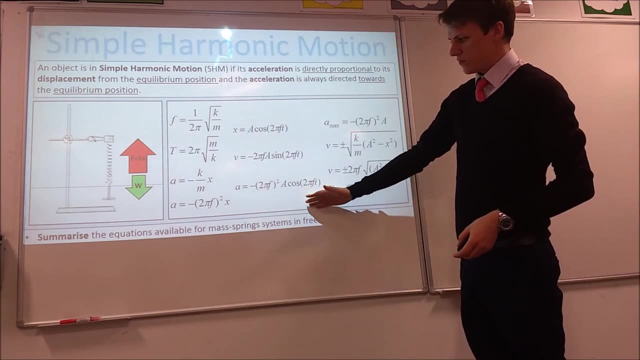 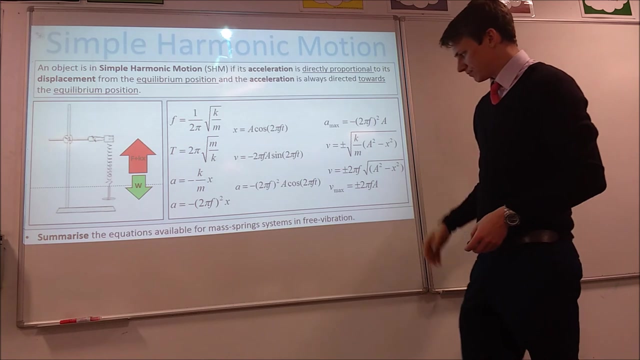 And, as I said earlier, look at transforming the equation we had for velocity in terms of displacement, Into what you'll see in your formula sheets. So these over here are the expressions we've derived already in terms of the acceleration and the natural frequency and time period. 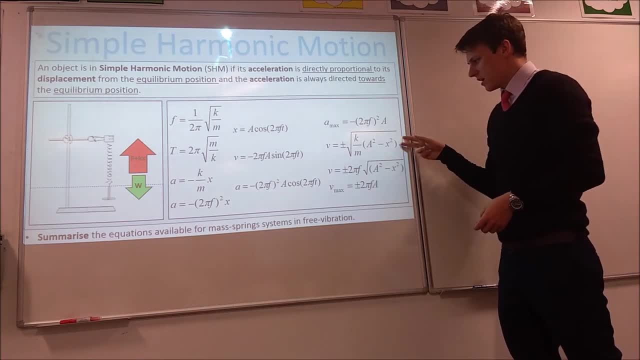 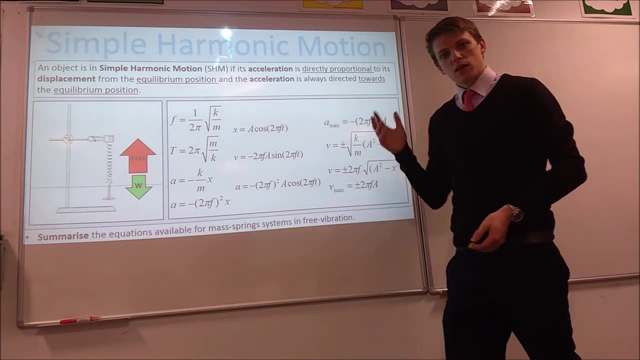 And this is the equation we derived for velocity earlier in terms of the displacement. So I said earlier, we're going to switch it around, So that's what we're going to do. So we've seen before that k over m is equal to 2 pi f squared. 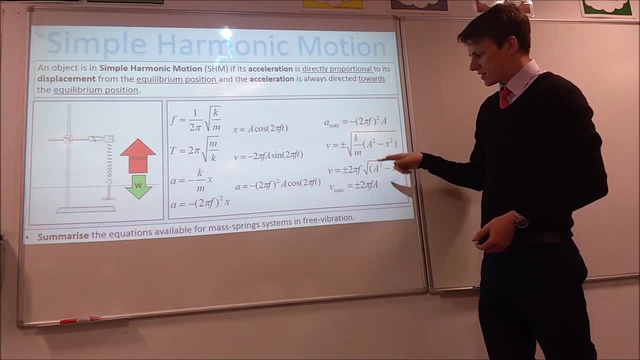 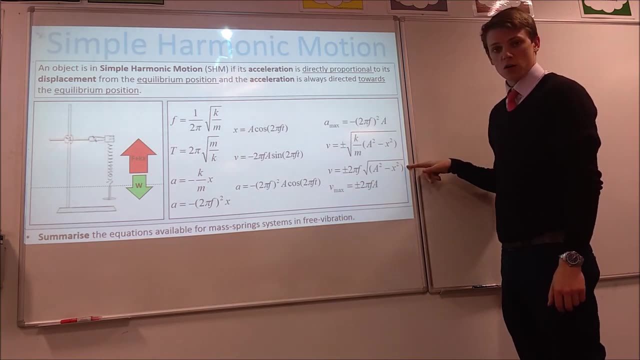 So we can substitute that That in for that, So we can then take it outside the square root because it's squared. So that's where we get this expression, which is usually in your formula sheet here in terms of the velocity there, Or sometimes you even see that written as an omega. 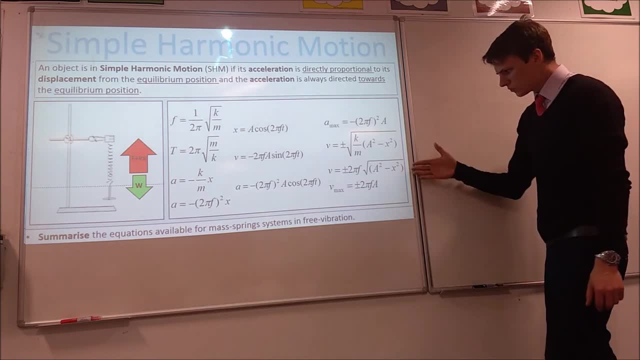 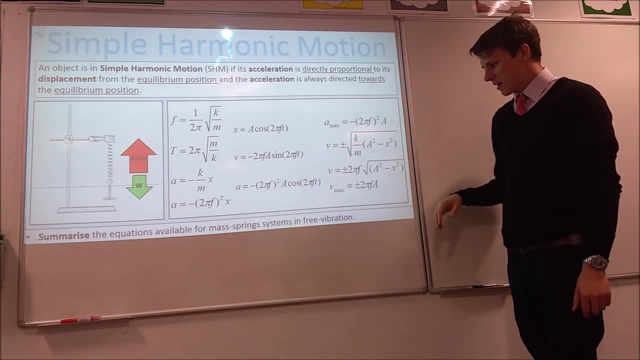 Those of you who've done circular motion will know where that comes from. So we can actually work out what the maximum velocity is in a cycle. So we can see from here. to get maximum velocity we need to make the displacement from the equilibrium position equal to zero. 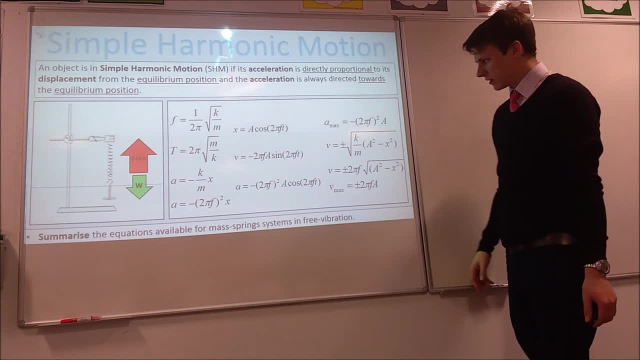 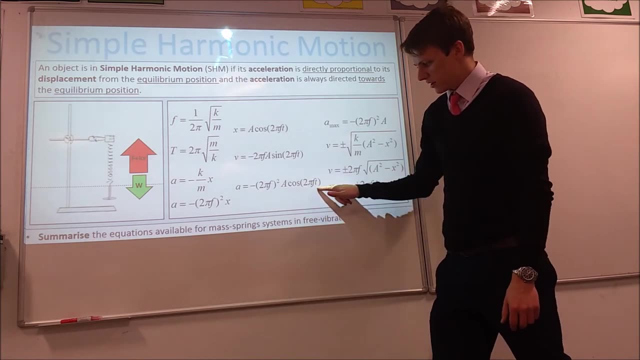 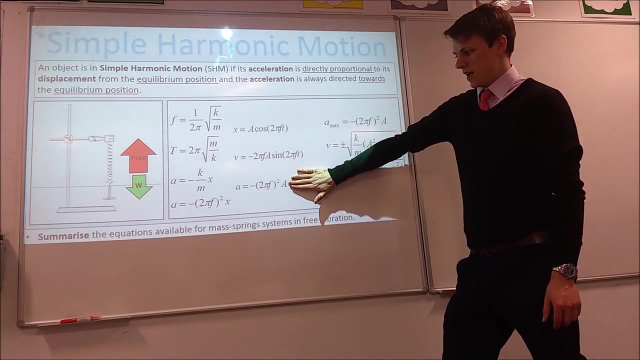 Because then we'll just get this expression 2 pi f- a. We can do a similar process for the acceleration here. So acceleration is maximized when this cosine function is going to be equal to 1.. So let's do that And we can see that we end up with maximum acceleration is 2 pi f squared a, multiplied by minus 1.. 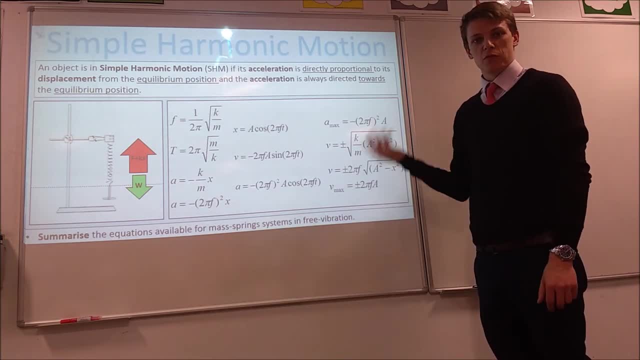 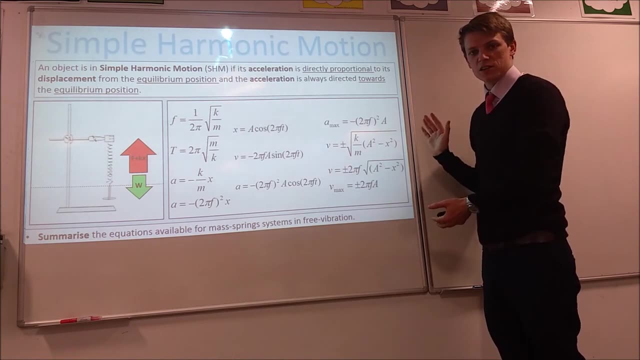 And that would then allow us to work out what the maximum force is in there which could be useful to us when we're modeling this system. So, when you're dealing with a matrix, When you're dealing with a math spring system, These are the equations you have to model how it's going to behave in different scenarios. 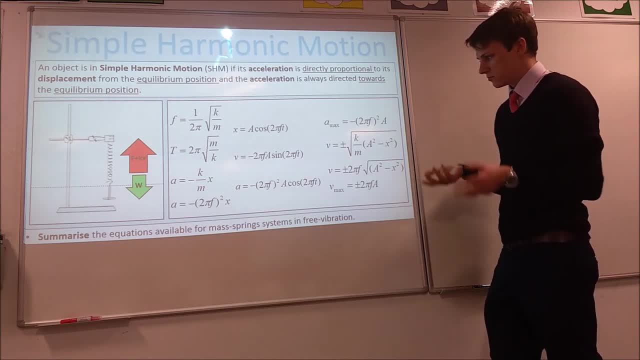 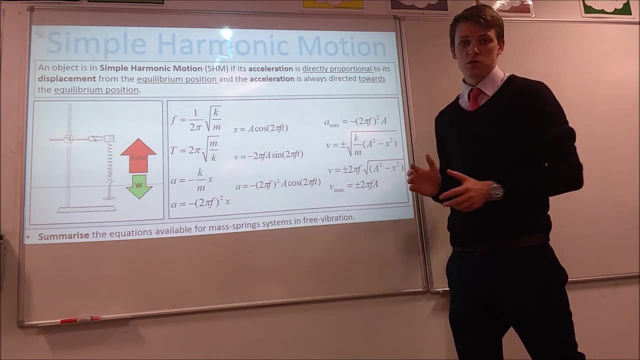 And this is what- or a slightly more complex version of this- people would use in modeling things like earthquakes, making musical instruments, all those kind of things. These are very useful for, And the last thing I just mentioned is the required practical. that's on this topic. 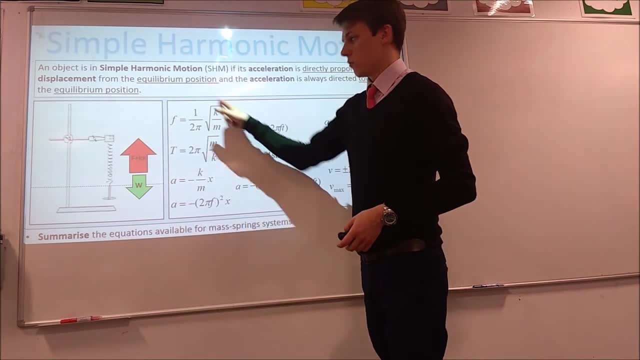 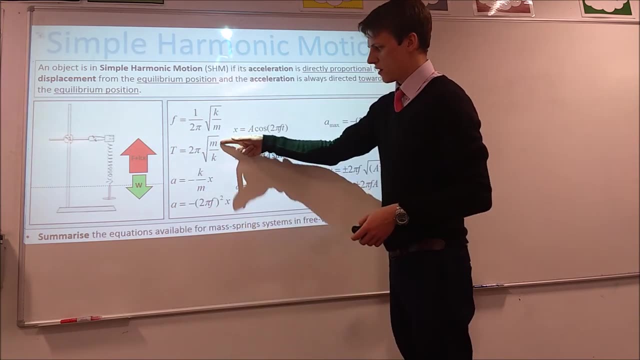 Essentially what you end up investigating. is this equation right here, or essentially the same as this one? You look at how different factors can affect the time constant of the oscillation. So varying mass, varying spring constant, those kind of things, And you'll see this relationship unfold.